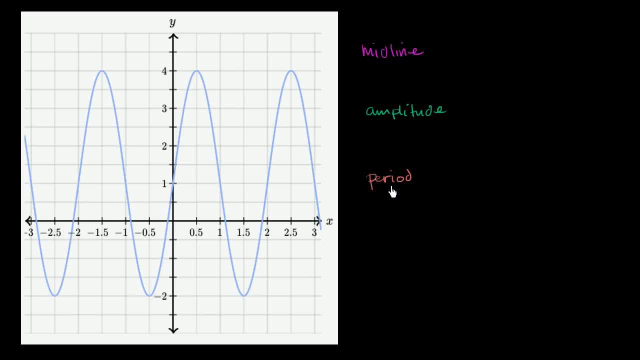 And then finally think about what the period of this function is. How much do you have to have a change in x to get to the same point in the cycle of this periodic function? So I encourage you to pause the video now and think about those questions. 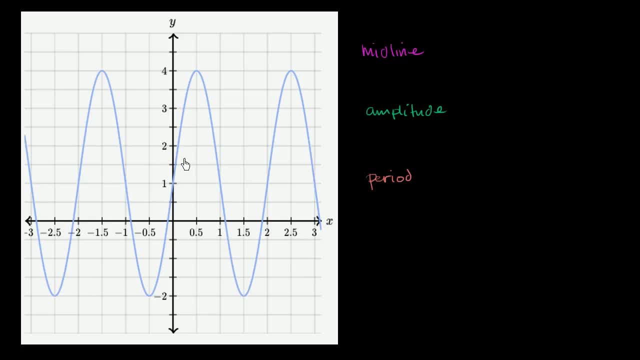 So let's tackle the midline first. So one way to think about it is: well, how high does this function go? Well, the highest y value for this function we see is 4.. It keeps hitting 4 on a fairly regular basis. 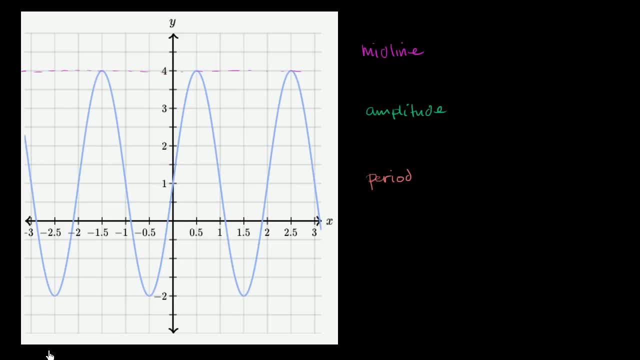 And we'll talk about how, How regular that is when we talk about the period And what's the lowest value that this function gets to. Well, it gets to: y equals negative 2.. So what's halfway between 4 and negative 2?? 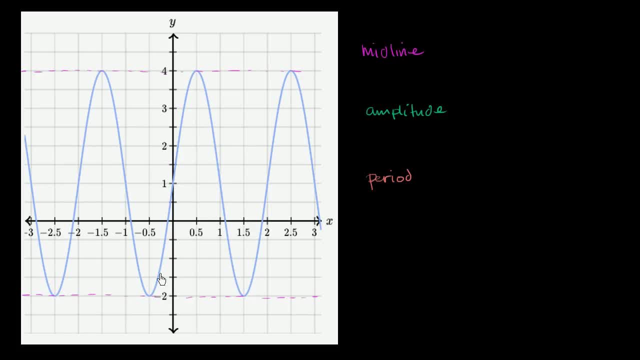 Well, you could eyeball it, or you could count, or you could literally just take the average between 4 and negative 2.. So the midline is going to be the horizontal line. y is equal to 4 plus negative 2 over 2, just literally. 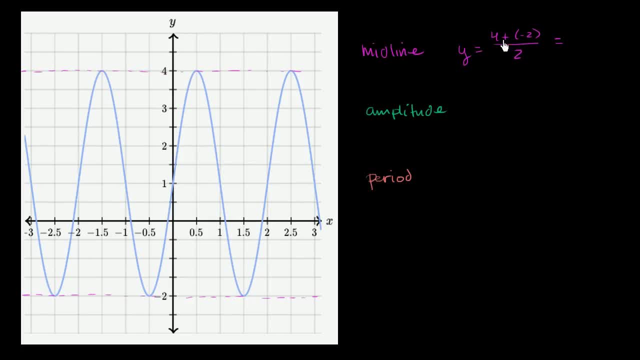 the mean, the arithmetic mean between 4 and negative 2, the average of 4 and negative 2, which is just going to be equal to 1.. So the line y equals 1 is the midline. So that's the midline right over here. 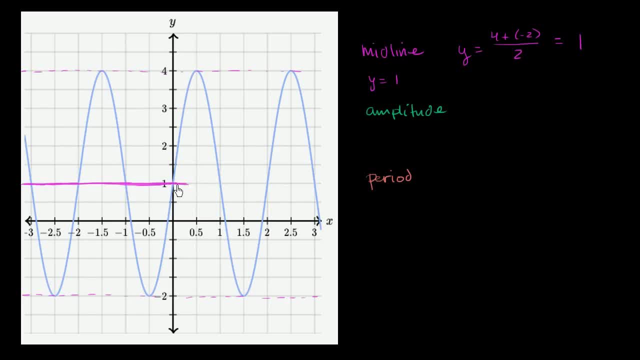 And you see that it's kind of cutting the function, where you have half of the function is above it and half of the function is below it. So that's the midline. Now let's think about the amplitude. Well, the amplitude is how much this function. 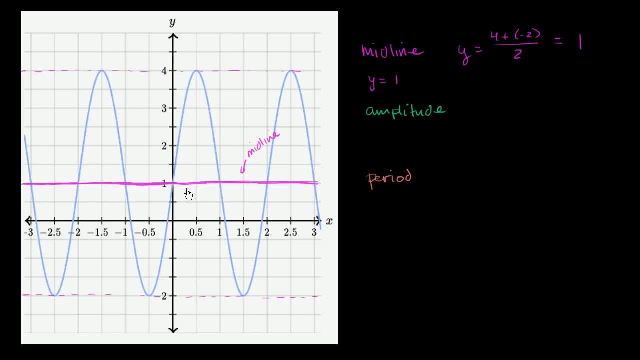 varies from the midline, either above the midline or below the midline, And the midline's in the middle. so it's going to be the same amount whether you go above or below. So one way to say it is: well, at this maximum point. 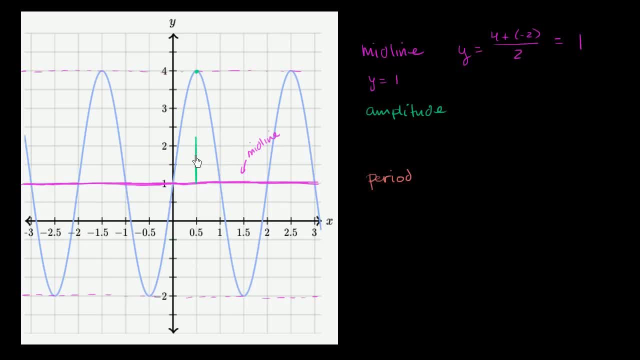 right over here. how far above the midline is this? How far above the midline is this? Well, to get from 1 to 4, you have to go your 3 above the midline, Or another way of thinking about it, this maximum point. 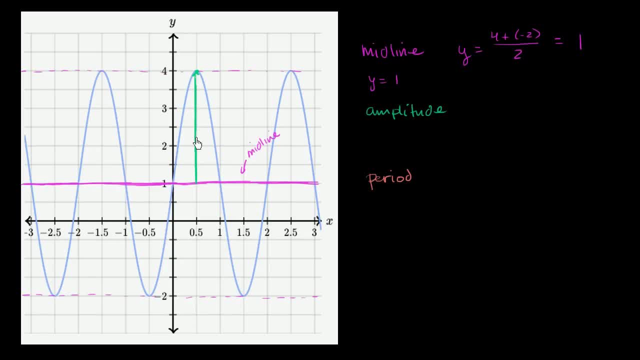 is y equals 4 minus y equals 1.. Well, your y can go as much as 3 above the midline. Or you could say your y value could be as much as 3 below the midline. That's this point right over here. 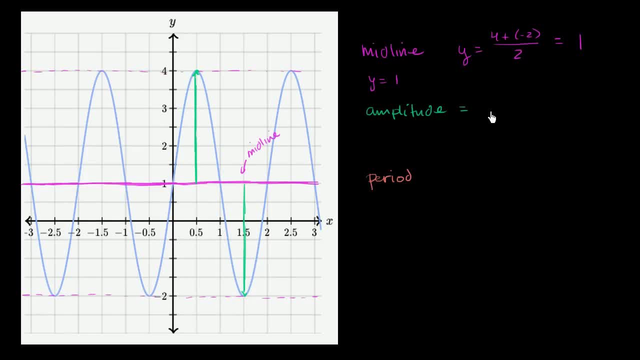 1 minus 3 is negative 1.. So your amplitude right over here is equal to 3.. You can vary as much as 3, either above the midline or below the midline. Finally, the period. And when I think about the period, 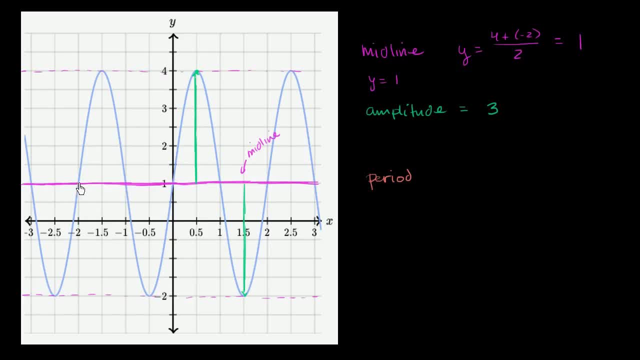 I try to look for a relatively convenient spot on this The curve, And I'm calling this a convenient spot because it's at a nice when x is at negative 2,, y is at 1,, it's at a nice integer value. 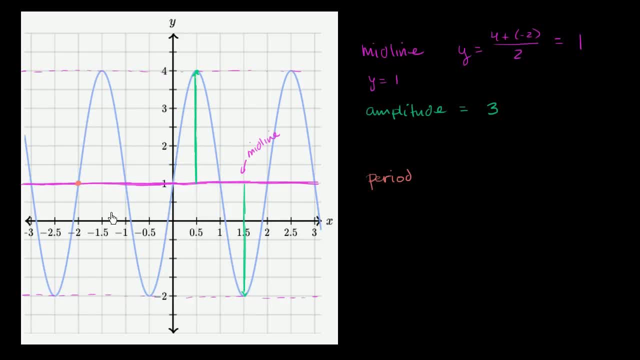 And so what I want to do is keep traveling along this curve until I get to the same y value, But not just the same y value, but I get to the same y value and I'm also traveling in the same direction. So, for example, let's travel along this curve. 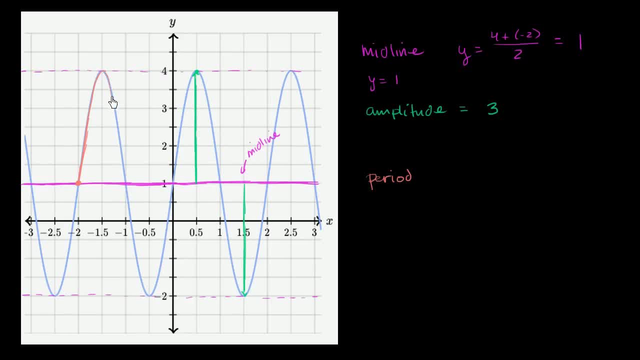 So, essentially, our x is increasing, Our x keeps increasing. Now you might say, hey, Have I completed a cycle here? Because once again, y is equal to 1.. You haven't completed a cycle here because, notice over here, our y is increasing as x increases. 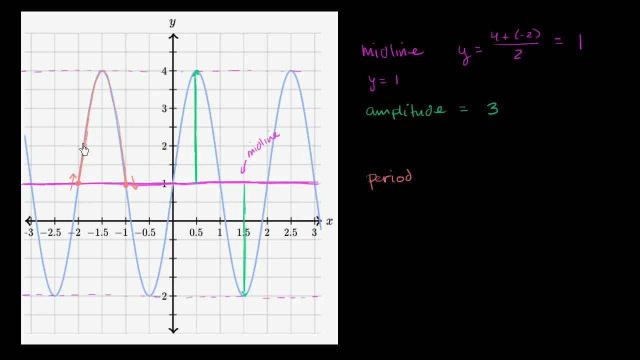 While here our y is decreasing as x increases, Our slope is positive here, Our slope is negative here. So this isn't the same point. on the cycle, We need to get to the point where y once again equals 1.. Or we could say, especially in this case, 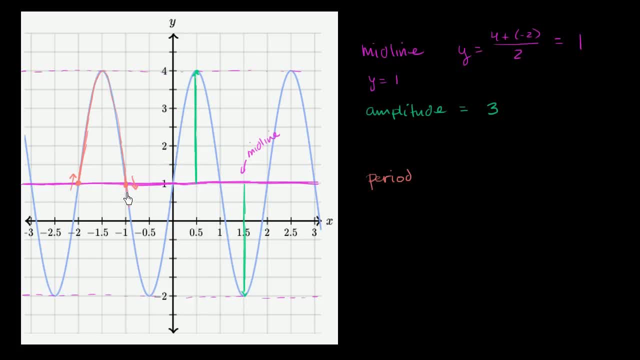 we're at the midline again, But our slope is increasing, So let's just keep going. So that gets us to right over there. So notice, now we have completed one cycle. So the change in x needed to complete one cycle. 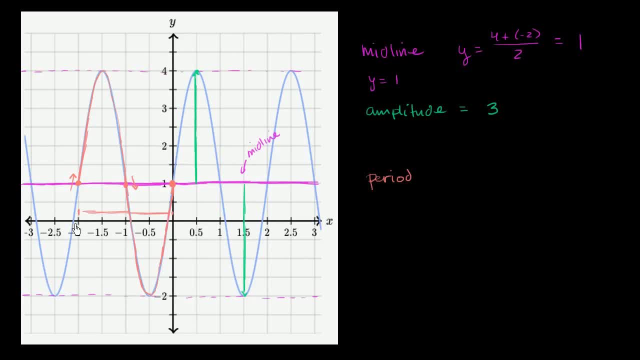 that is your period. So to go from negative 2 to 0,, your period is 2.. So your period here is 2.. And you could do it again. So we're at that point. Let's see, we want to get back to a point. 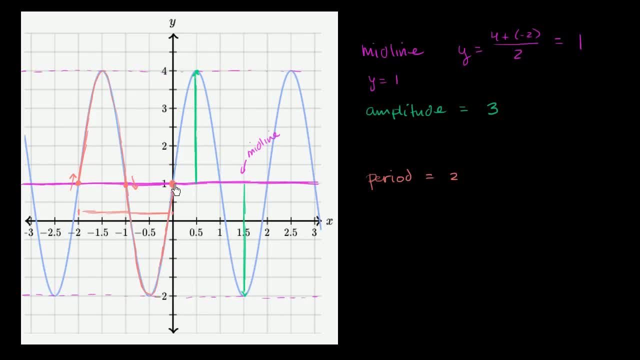 where we're at the midline And you know, I just happened to start right over here at the midline. I could have started really at any point. You want to get to the same point, but also where the slope is the same. 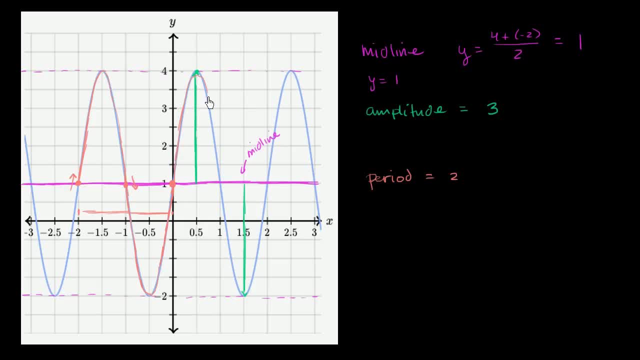 We're at the same point in the cycle once again, So I could go. So, if I travel 1,, I'm at the midline again, But I'm now going down, So I have to go further. Now I am back at that same point in the cycle.